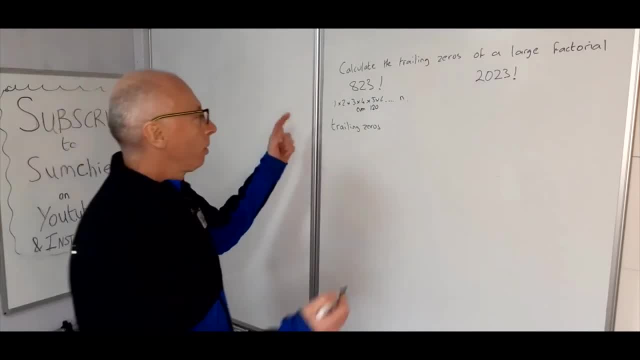 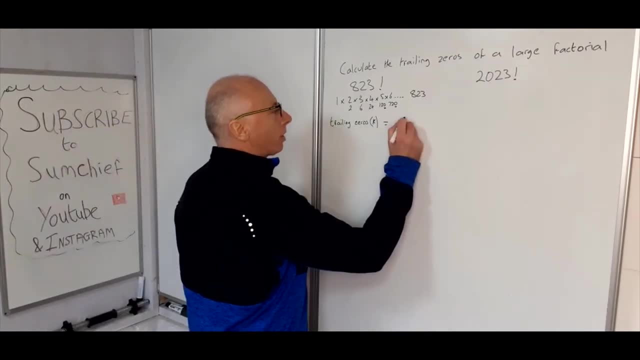 It's just a word, it's not a number. We can give it a letter if we like. We can just call it. for example, we'll call it k. Now there's a formula for it. So this summation goes from: x equals 1. 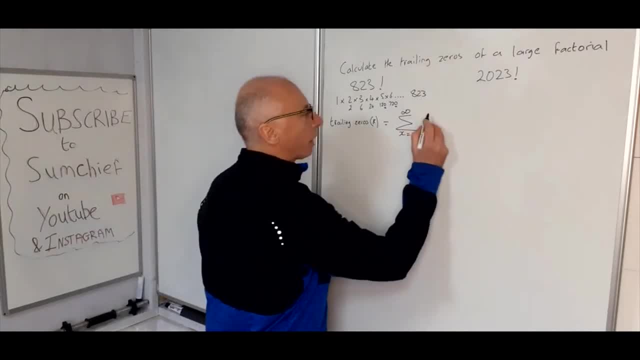 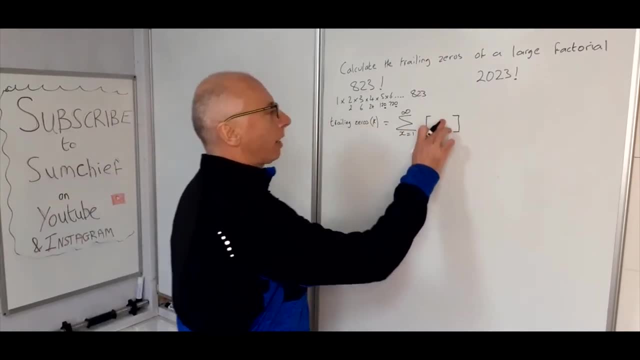 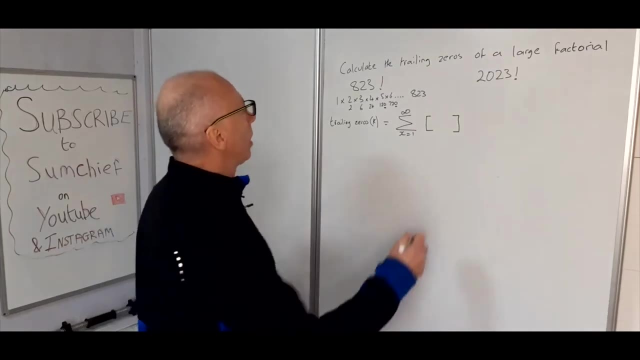 to infinity, and we're going to make use of the greatest integer function, which is open square bracket, close square bracket and then a number inside. Now the number inside here is going to be divided from a formula, So it's going to be n divided by prime number to the power of x. 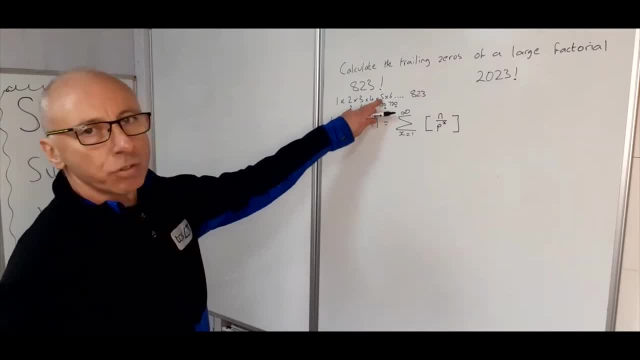 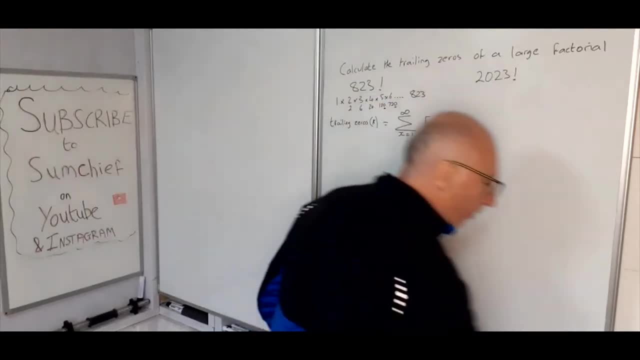 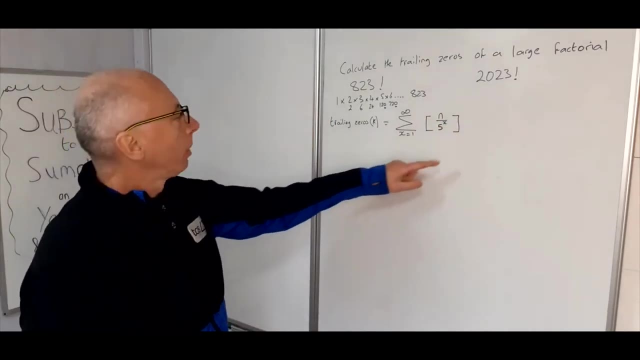 Now, because we're looking for trailing zeros and we're interested in five, we want this prime number to be five. So let's just change this p to be a five, because that's the only number we're interested in at the moment. Okay, and then we sum all these up and then we hopefully get the. 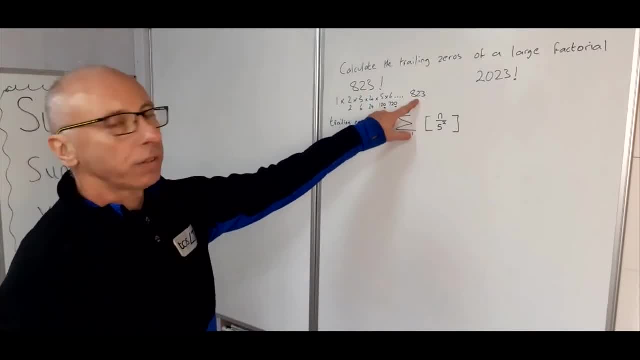 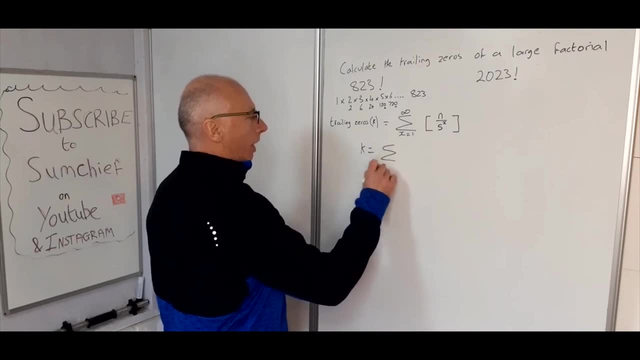 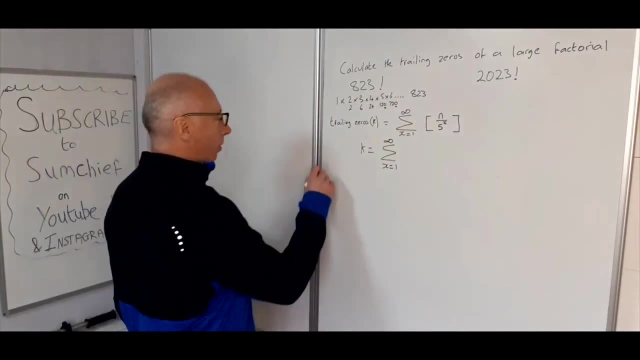 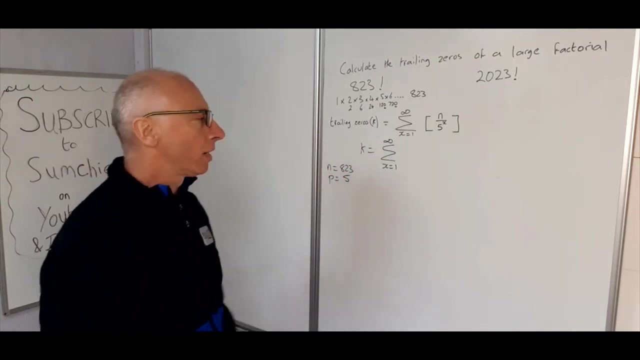 trailing zeros. So we're interested in 823 factorial. So let's just plug that in. So k equals x, equals 1 to infinity. Now our n in this case is 823.. So let's just write that down here. and the p is five. Well, we're only interested in five anyway, because it's trailing zeros. 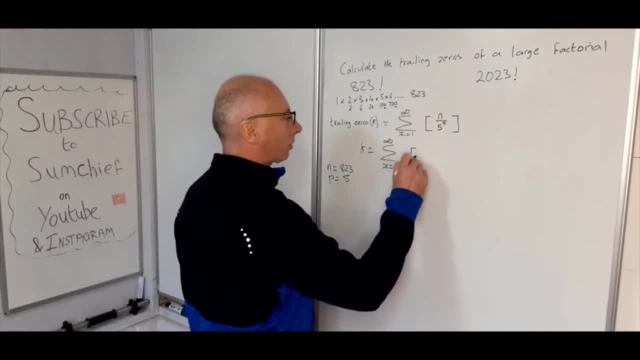 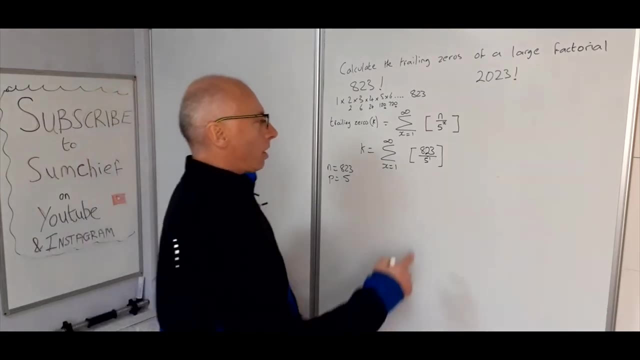 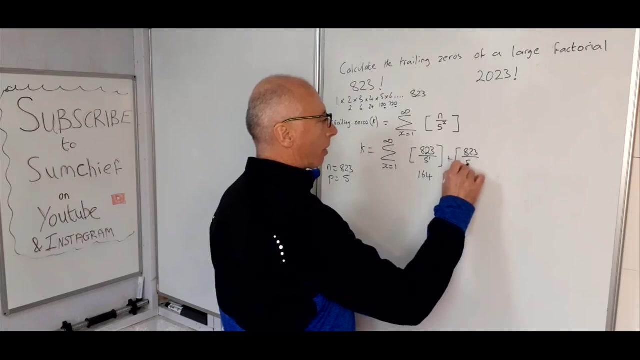 Okay so 823.. 823.. divided by five, to the power of one in this first case. So how many fives are there in 823?? Well, 165s are 800.. So that's going to give us 164.. Okay so now I want to: x equals two. So for x equals two, 823 divided by five, squared Now five. 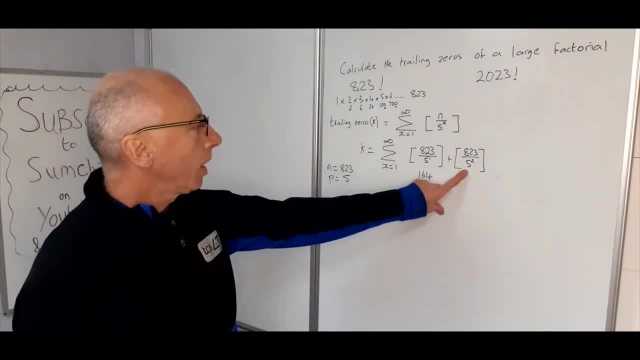 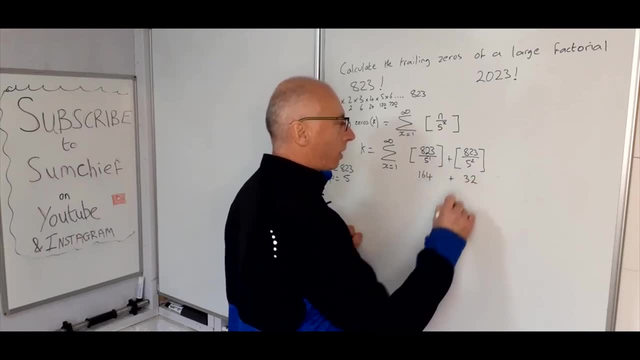 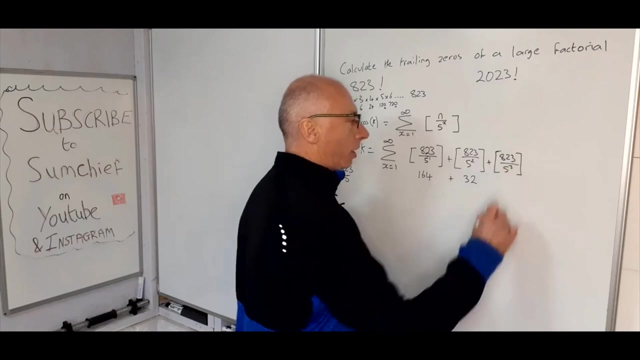 we know is 25.. So 25s into 823.. Four per hundred, So that's going to give us 32.. So that's our greatest integer function. Now it's 32 and a bit, but I was really interested in the whole numbers. Okay, so down to the next one: 823 by five cubed, So that's 125.. So how many? 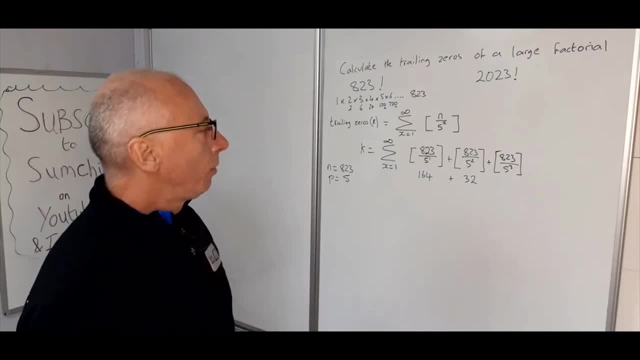 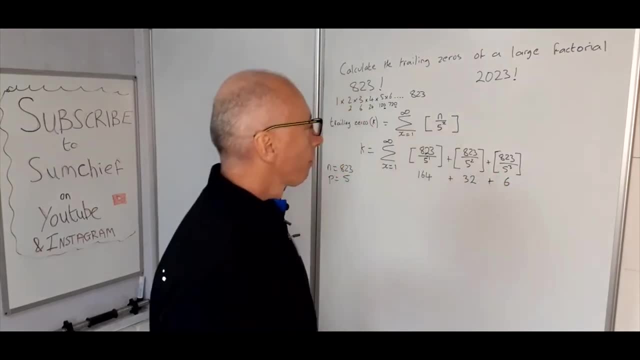 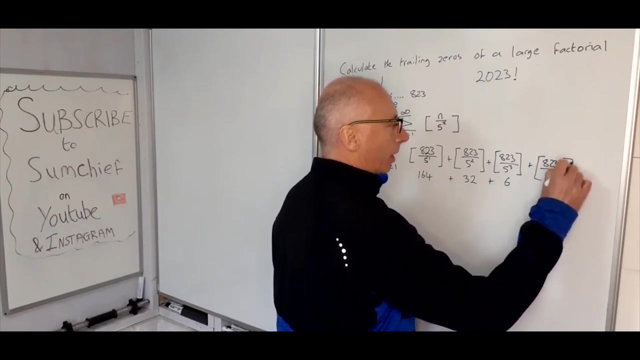 hundred and twenty-fives in 823?. The fourth would make 500. Six would make 750. So that's going to be six On to the next one. So got to go for all the possibilities. Five to the power of four, That's. 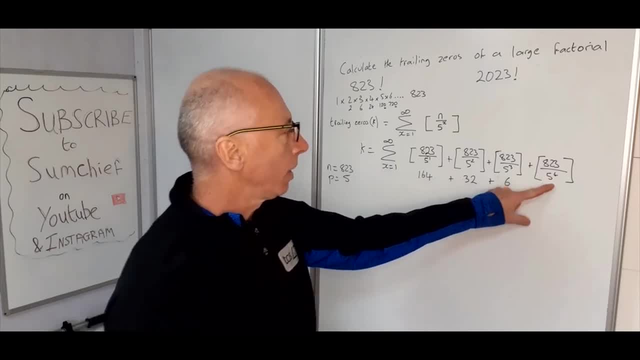 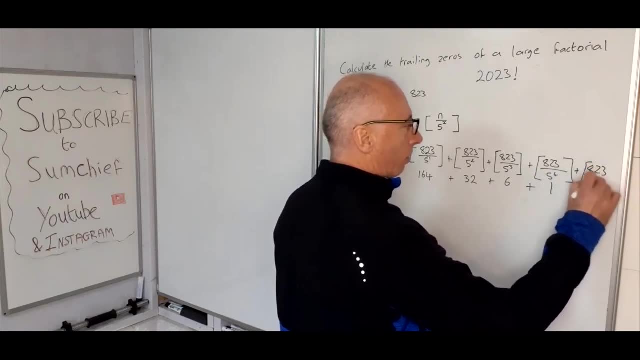 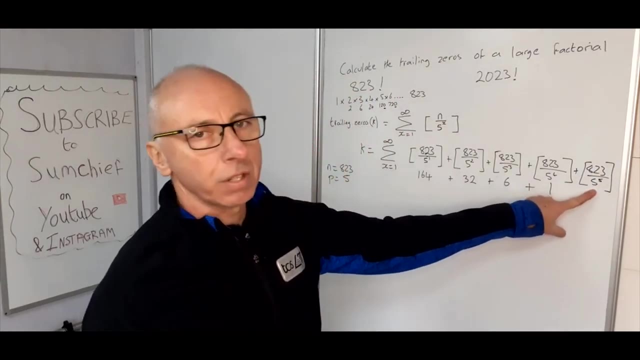 5 by 25, squared that 625.. So that's just going to give us one, And on to the next one: 823.. Five to three is six. power of 5, or 5 to the power of 5, is 625 times 5, which is 3125. so in terms of the 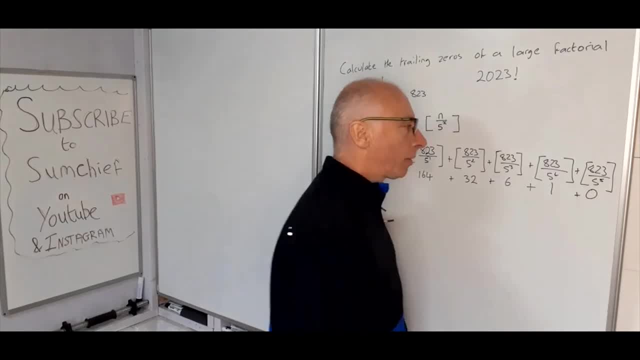 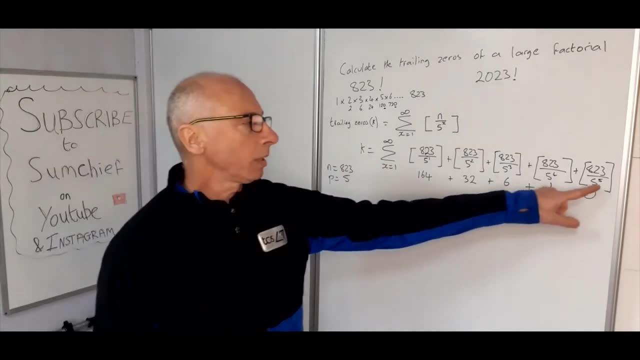 greatest integer function. this is just going to yield a zero. as we got to a zero here, with 5 to the power of 5 using the summation formula, we're not going to need to progress any further. so now what we need to do is just add up this: these: 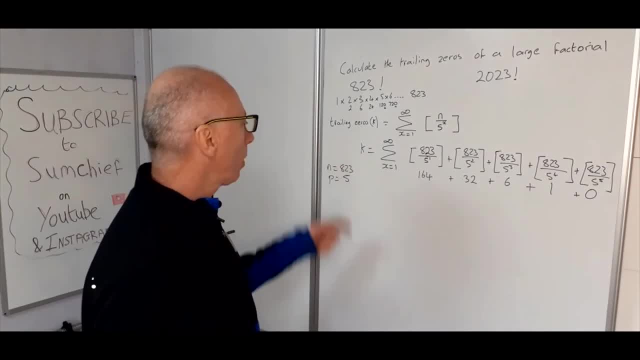 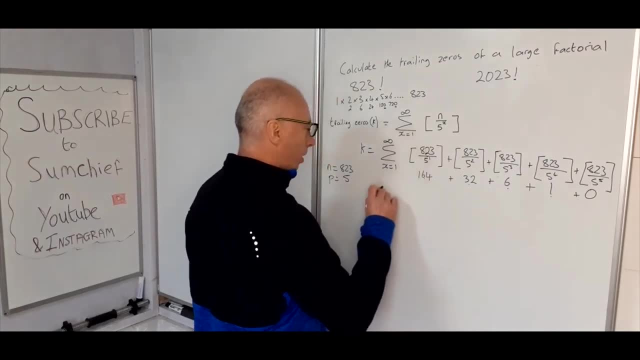 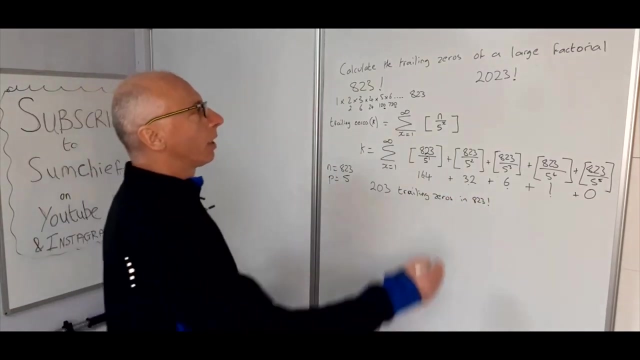 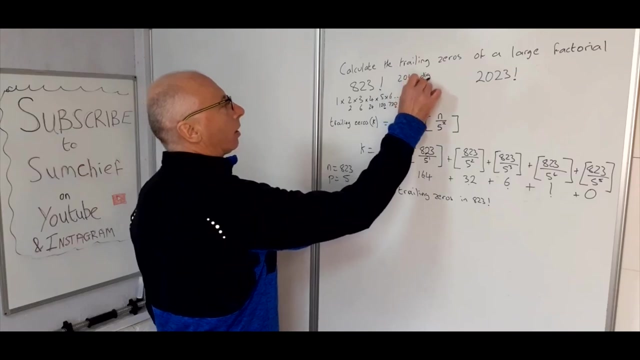 numbers here and that will give us our trailing zeros in 823 factorial. so 164, 196, 202, 203. so therefore we can say there are 203 trailing zeros in 823 factorial. so if you write that number out, I think I said 2044 digits for 823. 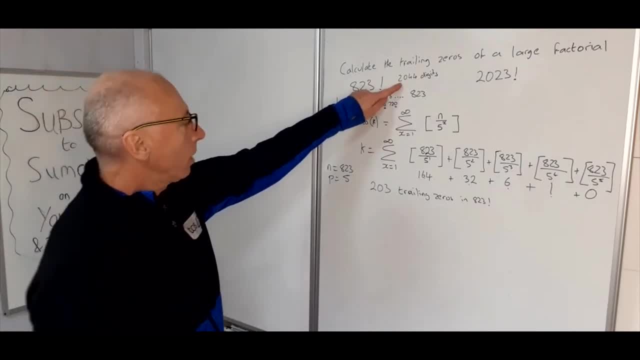 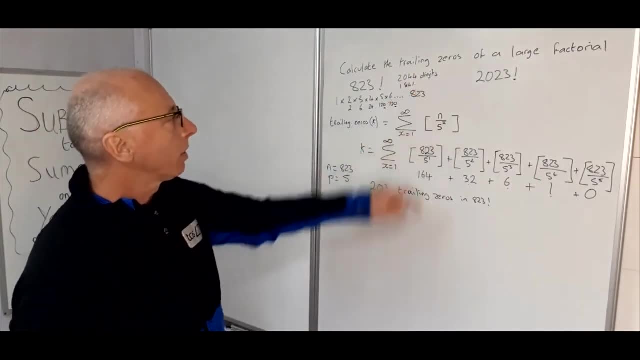 factorial. so if you write that number out- I think I said 2044 digits for 823 factorial, so you would get to 1841 and then after that all you'd be writing will be zeros to get to the end of the 2044. okay, so that's how we work out 823 factorials. 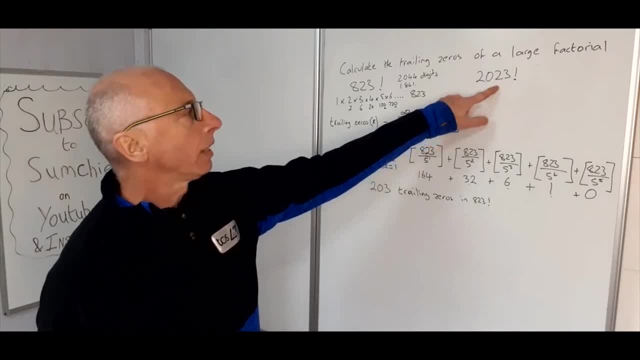 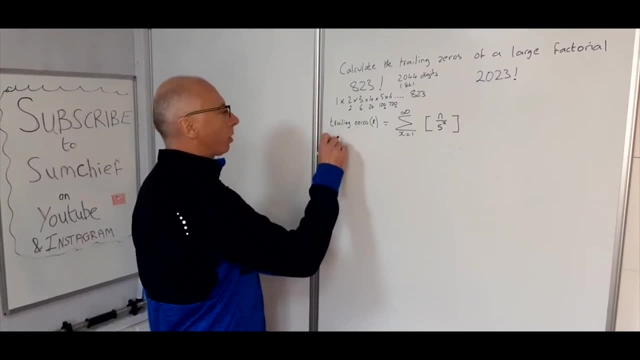 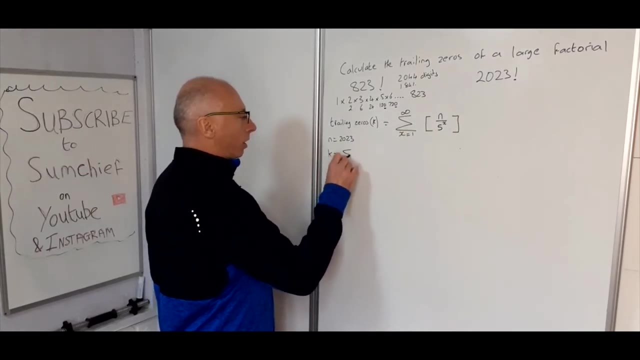 trailing zeros. so now let's move on to 2023. okay, so for 2023, now we've got our n equals 2, 0, 2, 3 for this formula. so then we want: k equals the sum of x equals 1 to infinity. 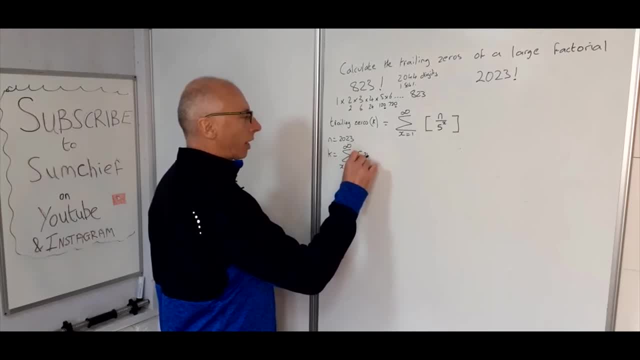 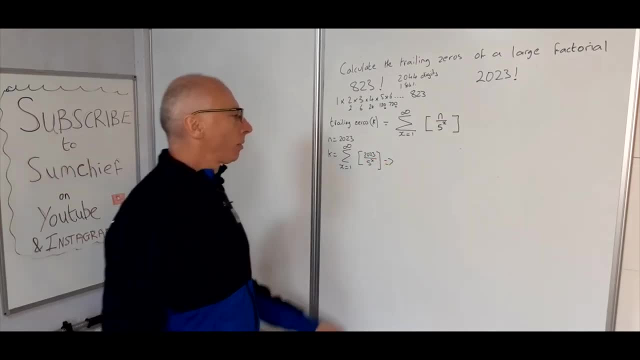 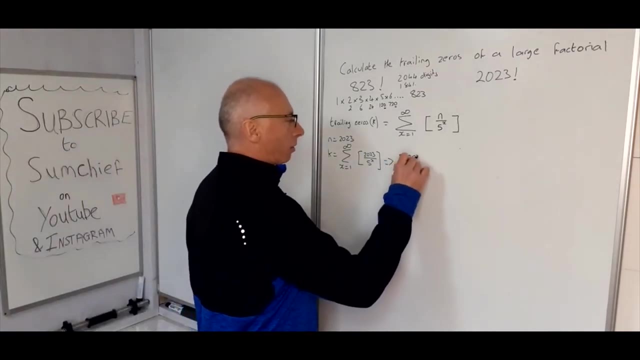 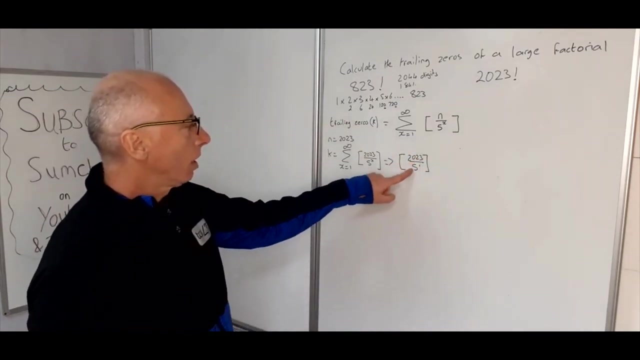 greater integer of 2023, 5 to the x. so then, this is going to lead us to, so just go through. the x equals 1, 2, 3, 4 and so on. so 2, 0, 2, 3, 5 to the power of 1. so how many 5s into 2023? well, 400 5s. 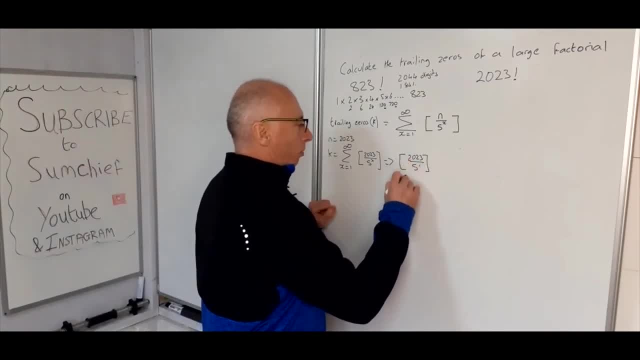 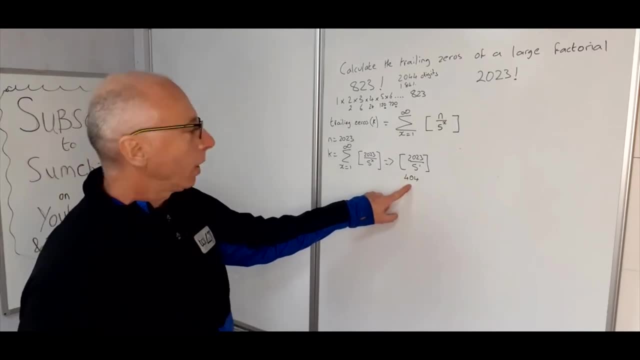 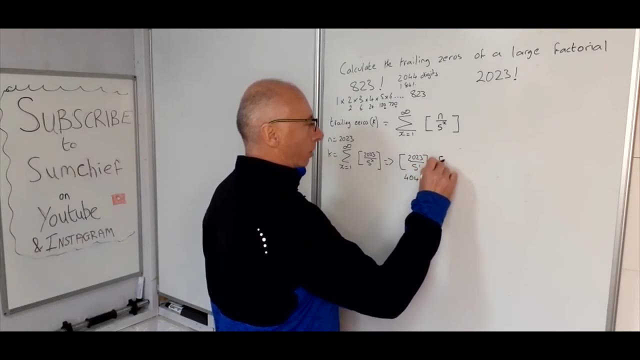 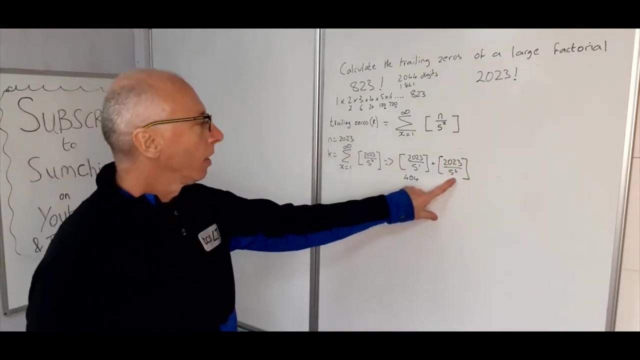 is 2000, so 404 will be 5, 5. so you multiply 5 by 404, we get 2020, and then that will give us our lowest value that we can do. that's a whole number. and then we've got 2: 0, 2, 3, 5 squared. well, that's 5 squared 25, 4 per 100, and we've got 20 of those. 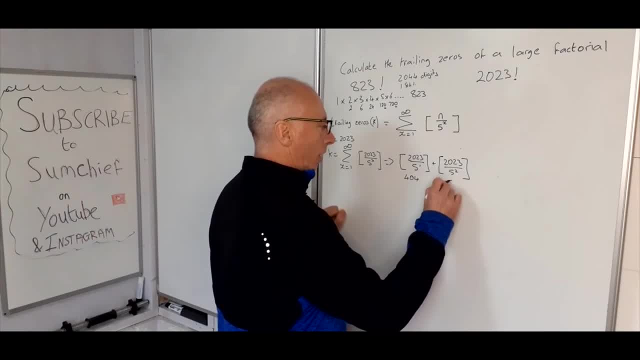 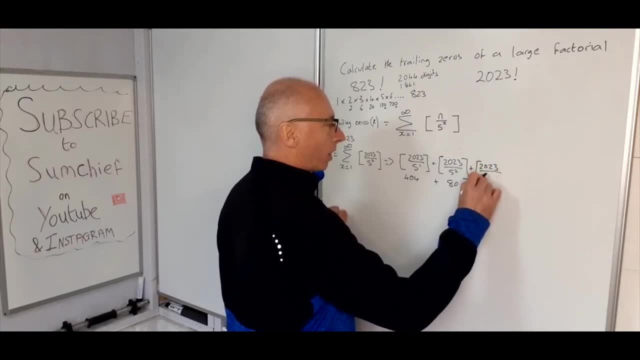 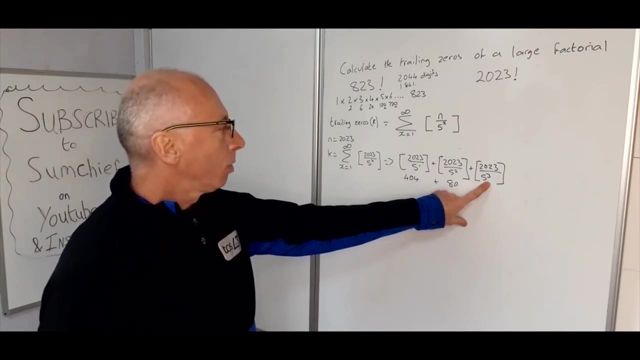 that's going to give us 80. that's then i'm going to give us 80. okay, we might run out of space on the side here. 2023: 5 cubed. 5 cubed is 125. now there's 8 125s. 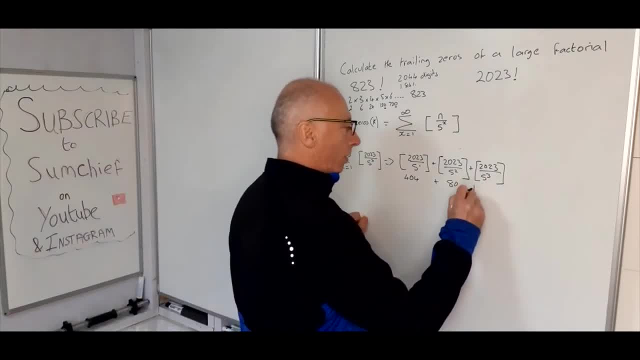 per 100 and we've got 20 of those, that's going to give us 80. that's going to give us 80 per 100, so that's then going to give us, as it's 2023, it's going to give us 16.. 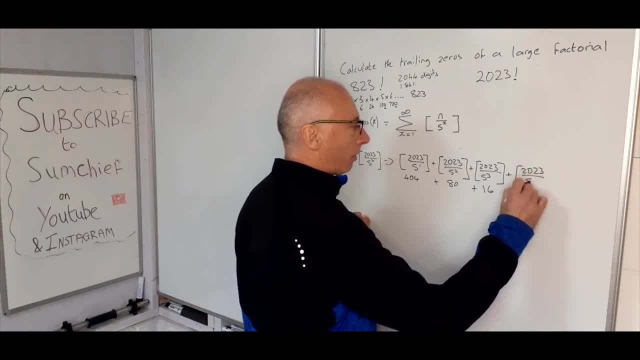 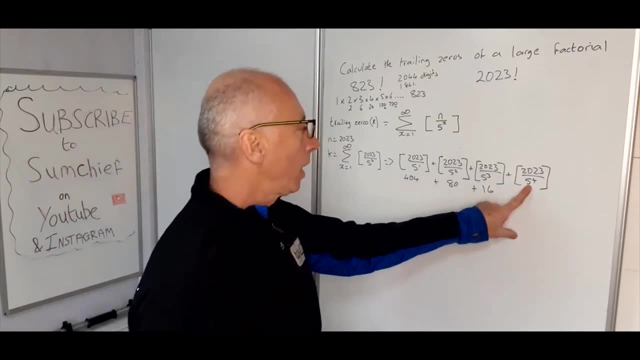 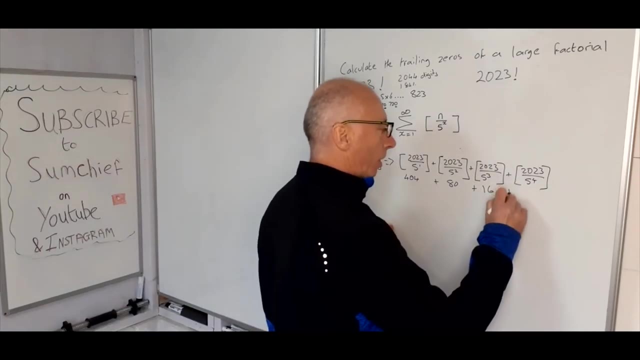 okay, 2023: 5 to the power of 4.. 5 to power 4 is 625, that's 25 squared. so 625 cubed is going to give us 1875. so that will give us our greatest integer value for that one. now i'm thinking. 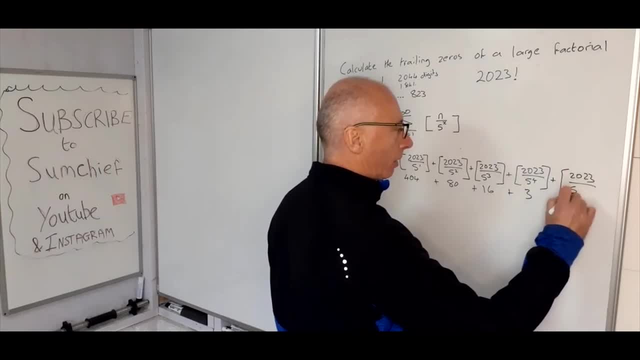 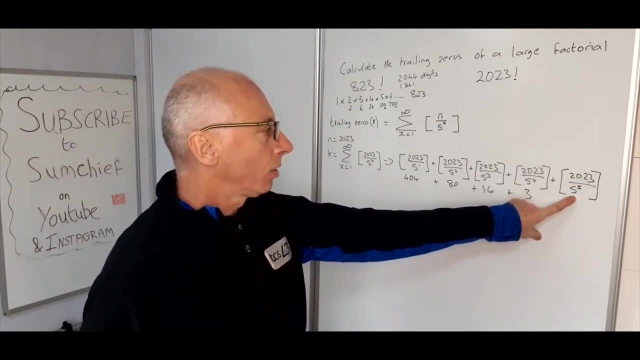 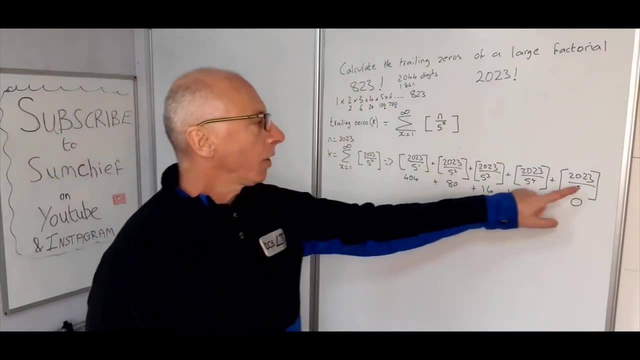 this one is probably going to be our last one on here. 5 to the power of 5. 5 to the power of 5 is 3125, so this is going to give us a 0, and as our x is only going up to five, and we get a 0, we don't need